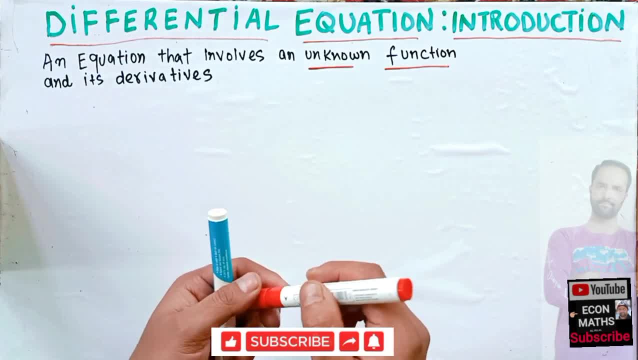 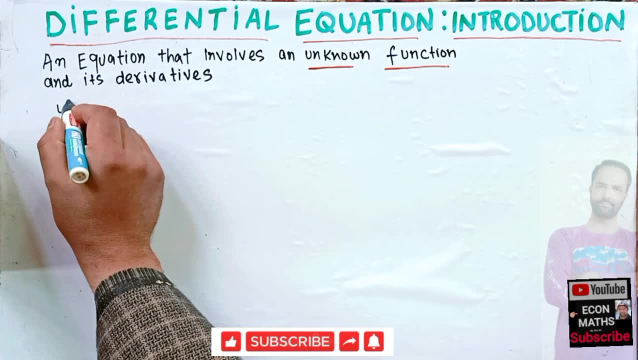 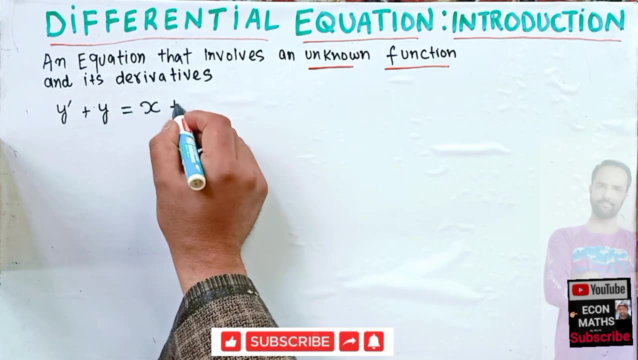 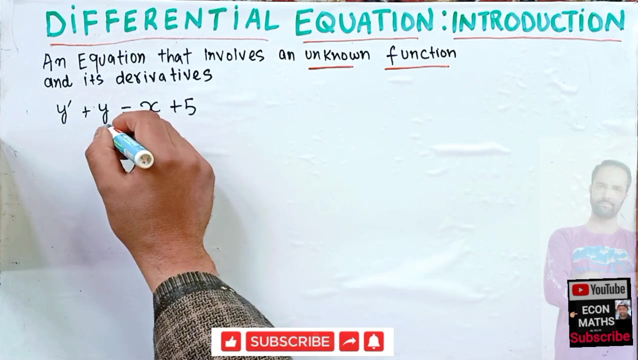 unknown function and its derivative or derivatives. Okay, one or more derivatives. Let's write it like this: We have, let us say we have- a function: y prime plus y is equal to x plus 5.. Okay, this is a sort of differential equation. Okay, here we have this unknown function. 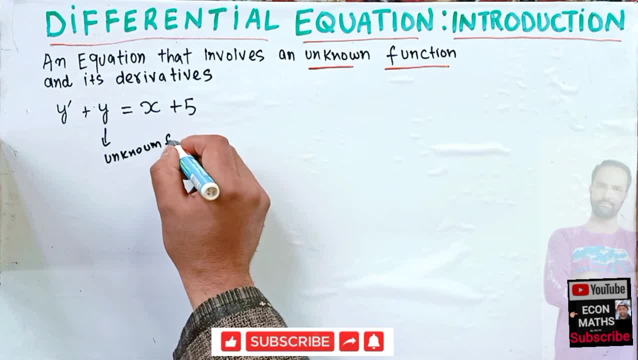 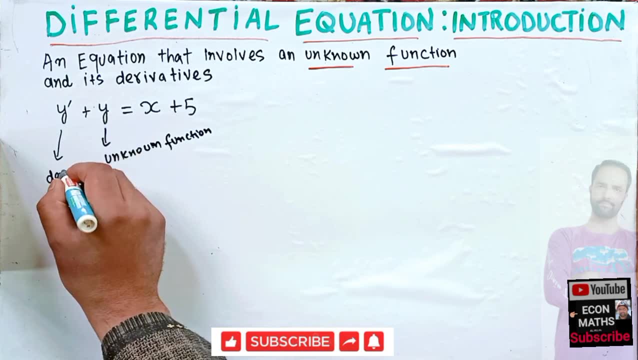 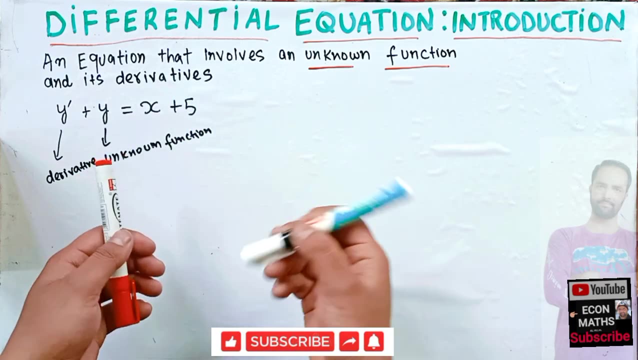 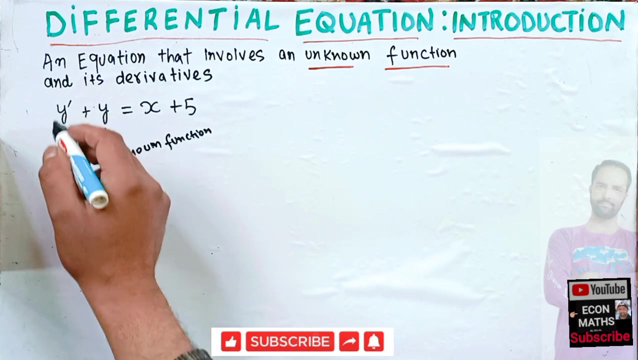 We have this unknown function, Okay, and its derivative. That is derivative, Okay. so simple thing. An equation that involves an unknown function and its derivative is called a differential equation, And this can be written in another way. We have another terminology. We can write it like this: dy upon dx plus y is equal to x plus y. 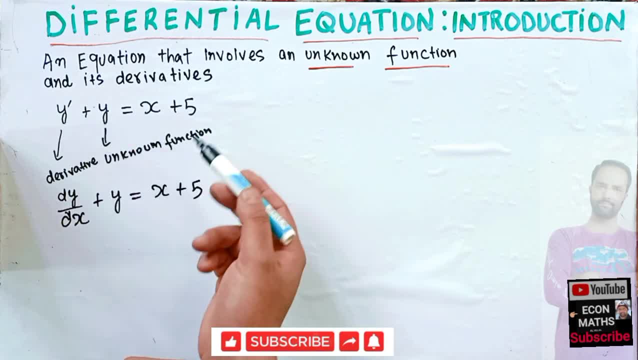 Whether you write in this notation or in this notation, these both give us same meaning. And we can also write it like this: f dash x plus f of x is equal to x plus 5.. Okay, these three denote same equations and they are the differential equations. Now there might be the question in: 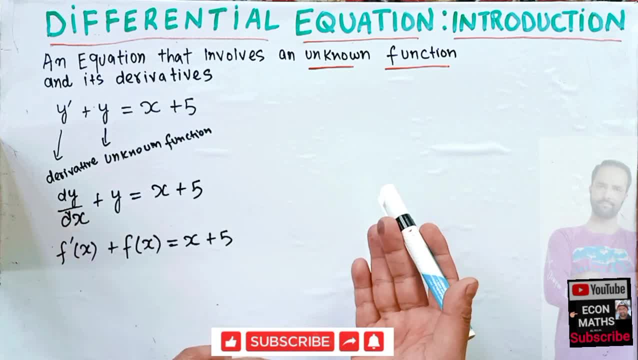 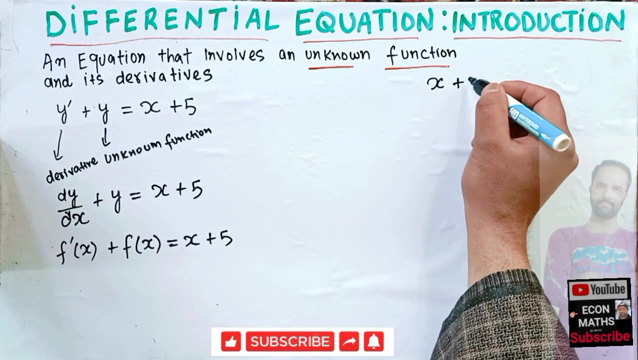 your mind Now how it is different. So let's try to see what is our regular equation. We can have an equation which we often use, The regular equation like this: x plus- let us say we have x plus 2- is equal to 0. Okay, 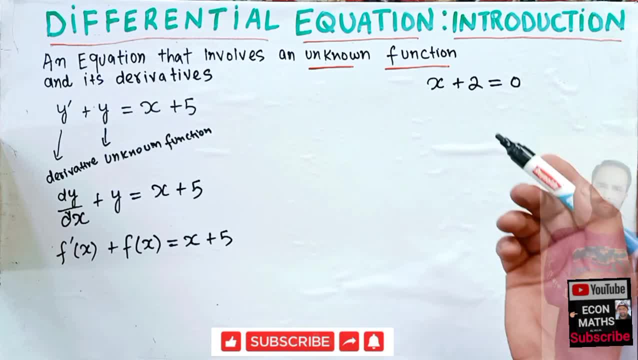 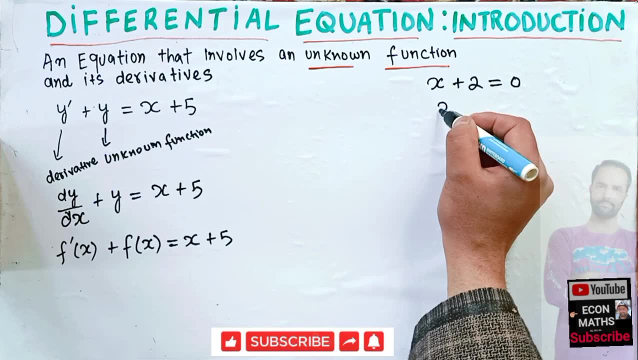 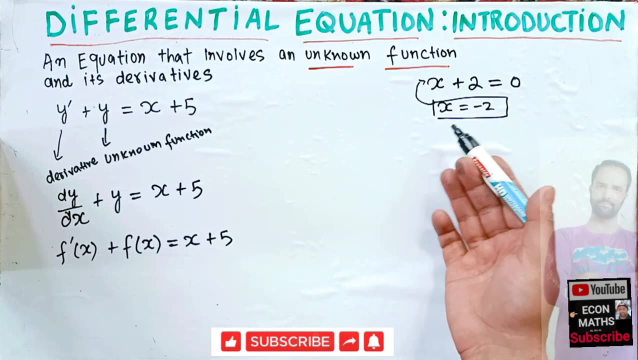 this is our regular equation. Here you can say this is an algebraic equation. The solution of this regular equation can be found as simply if we set it equal to x plus y. So let's try to see if this is equal to minus 2.. We say that the solution of this regular equation is minus 2.. Okay. 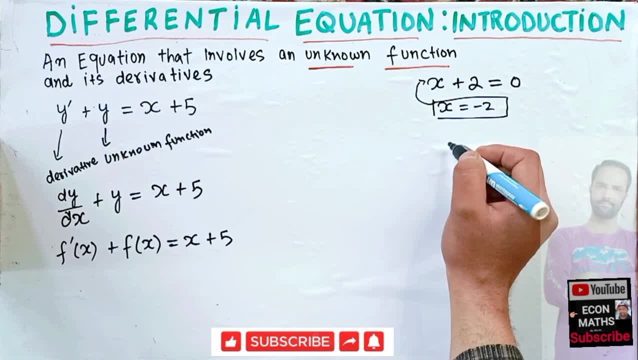 or if we have another equation, let us write it like this: This is our regular equation. And let's write another equation. Let us say x square minus 5x plus 6.. Okay, and what will be the solution of this regular equation? So we can see here: if we factor this out, we will get. 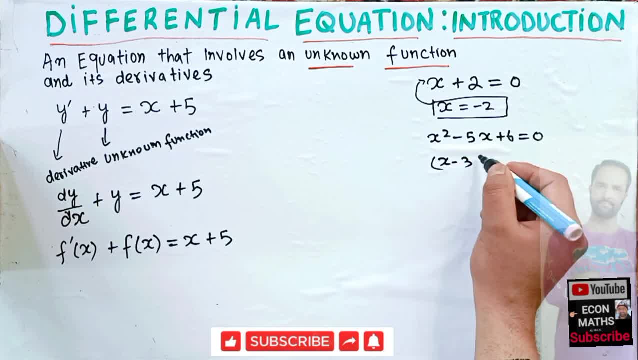 x minus 3 into x minus 2 is equal to 0, which means the solution to this equation will be: either x is equal to minus 3 or- sorry, plus 3.. If I let's write it here, The solution will be x. 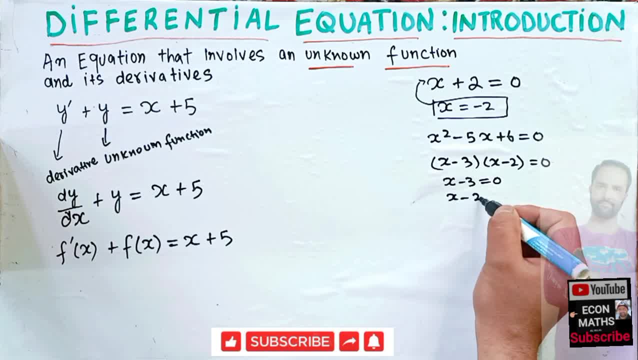 minus 3 is equal to 0 or x minus 2 is equal to 0, which gives us the solution is: x is equal to 3.. And x is equal to 2.. Okay, we get two solutions, two numbers as a solution of this equation. Now, 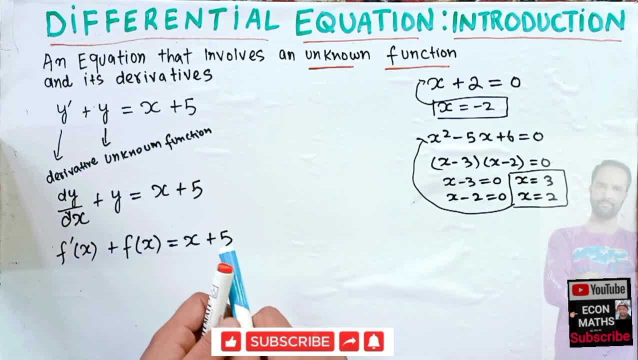 the difference between a differential equation and a regular equation is simply that the solution of a differential equation is a function, not a number or set of numbers. Okay, so the basic difference between what we call a differential equation is a function, not a number or set of numbers. 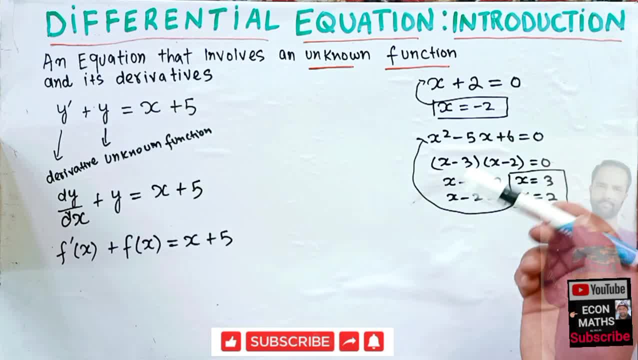 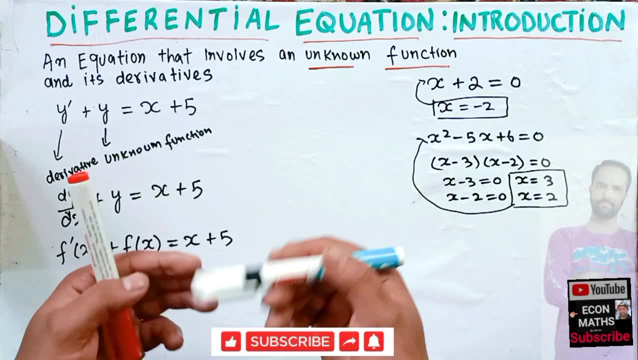 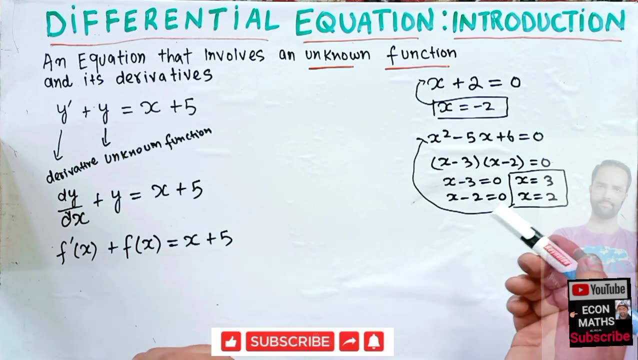 Between this differential equation and the regular equation is that in case of the differential equations, the solution is simply a function or a set of functions or a class of functions. Okay, so in the regular equations we get a solution as numbers or set of numbers. Okay, here we got two. 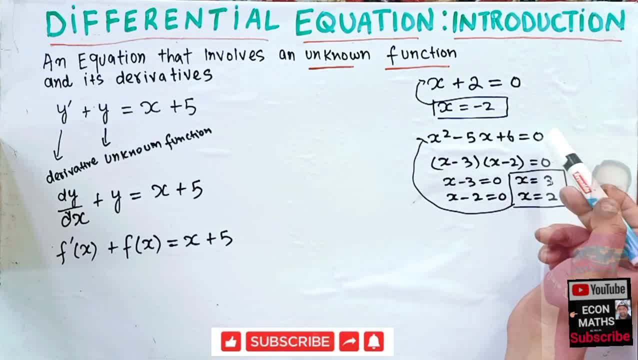 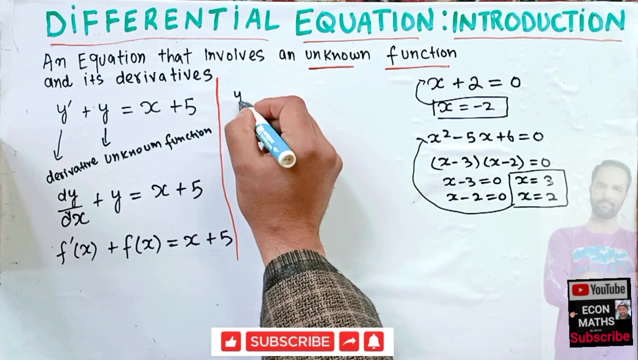 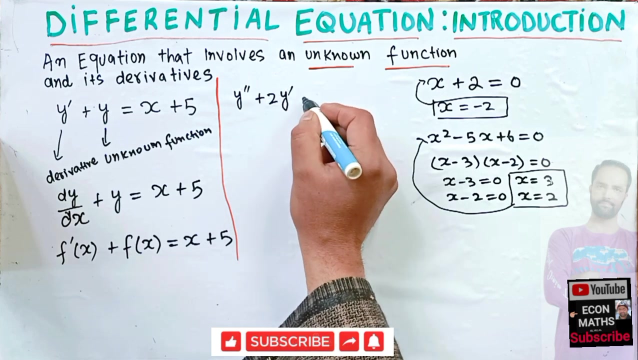 solutions to this quadratic equation. Okay, and here we got only one solution to this. Okay, so let us write a differential equation. So let us check it out also. So let us say we have a differential equation of, like this: y double prime, that means secondary derivative plus 2 y prime minus 3 y is equal to. 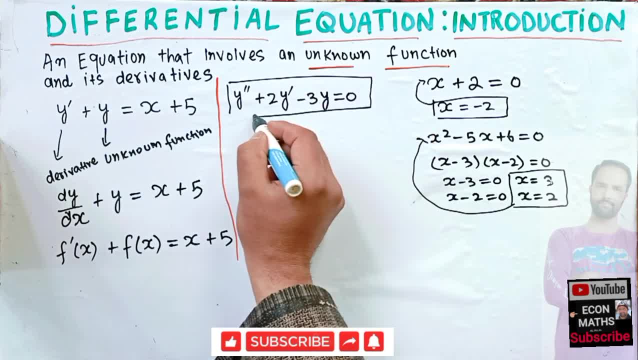 0.. This is our differential equation. Okay, its solution will be okay. so the solution of this equation, this we call the differential equation- is, let us write it like this: y 1 of x is equal to e to the power. 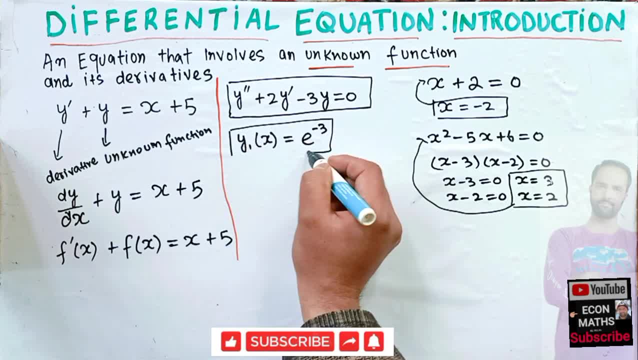 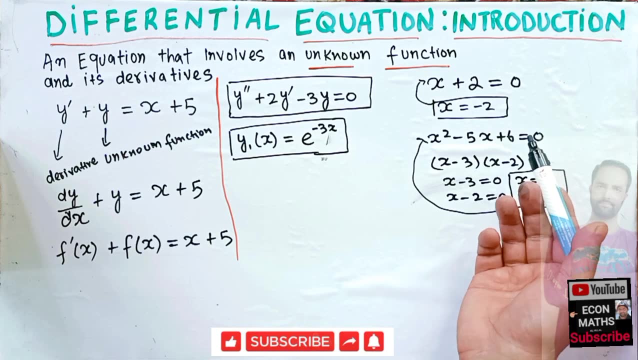 minus 3 x. I am saying the solution of: obviously we have here 3 x. Okay, so the solution of this differential equation is a function, not a number. Okay, its solution is a function. So how did I get this very thing, the solution of a differential equation? I will explain this. 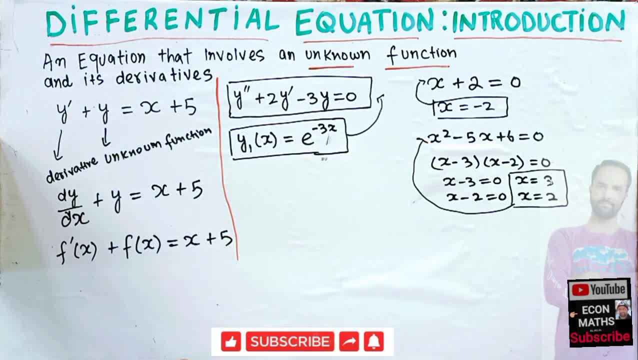 how do I get this very stuff? I will explain in preceding videos how did I get, but here I want to make. the point that I want to make here is that the solution of a differential equation is a function or a set of functions. Okay, now how do we verify whether this very stuff is the solution? 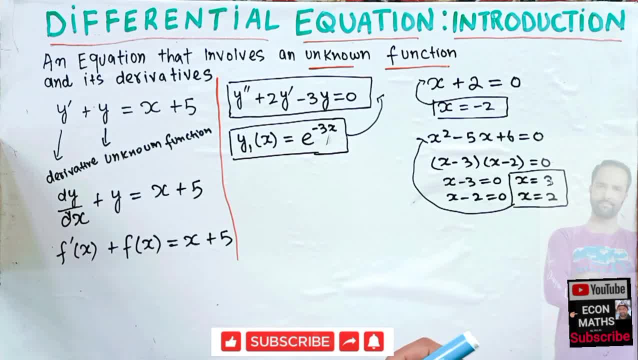 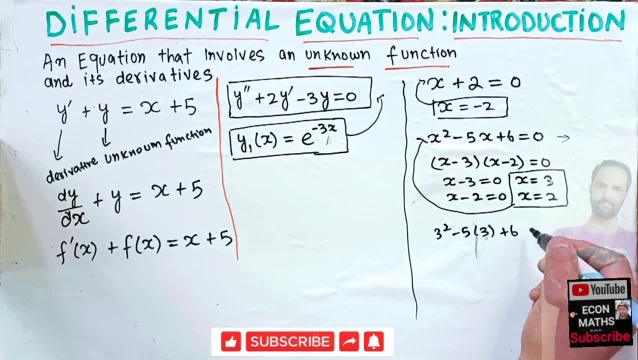 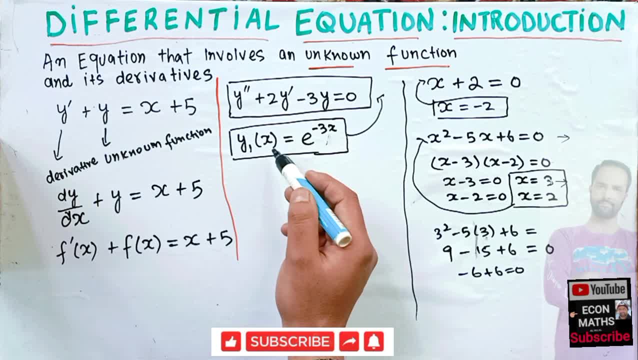 up. Okay, similarly, to verify whether this y 1 x is equal to e to the power minus 3 x is the solution of this differential equation. we just plug. the value of y 1 x is equal to e to the power x in this equation. Okay, in the. 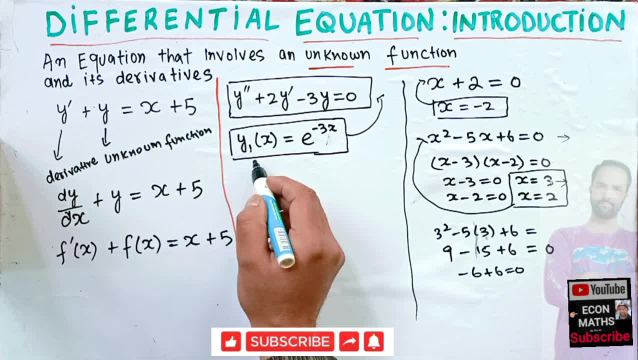 differential equation. Let's see. So we have y 1 x is equal to e, to the power, minus 3 x. okay, now that means y 1 prime x. that means this very stuff. so what will be y 1 prime x? so simply differentiate this function with respect to x will give us y 1 prime. okay, so we. 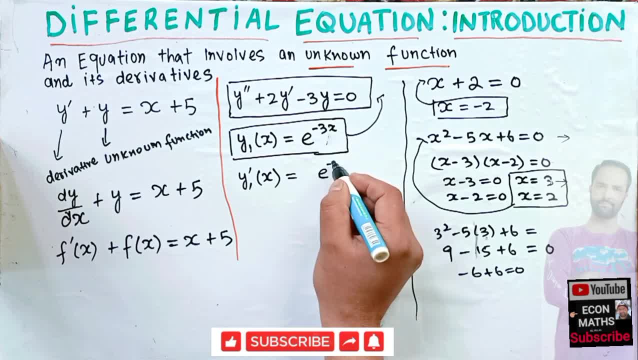 have e to the power, 3, x. so the exponential function and its derivative, simply the given function and the derivative of minus 3 x, and it is multiplied to this exponential function. okay, this is from the rule of differentiation. so we have here minus 3. okay, so we got y, 1, prime is: 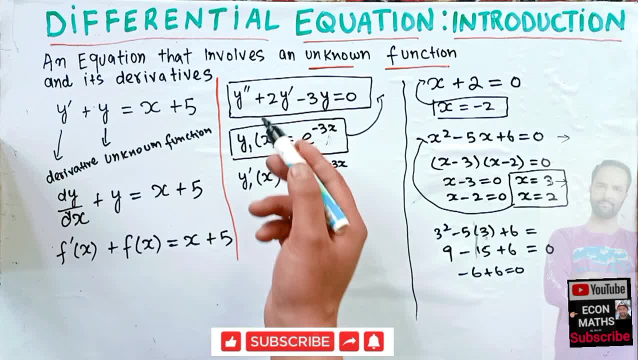 equal to minus 3 e, to the power minus 3 x. now what is y double dash prime? so let us write it like this: y 1 double dash prime of x. that means we need to take secondary derivative of this function. okay, so how do we? 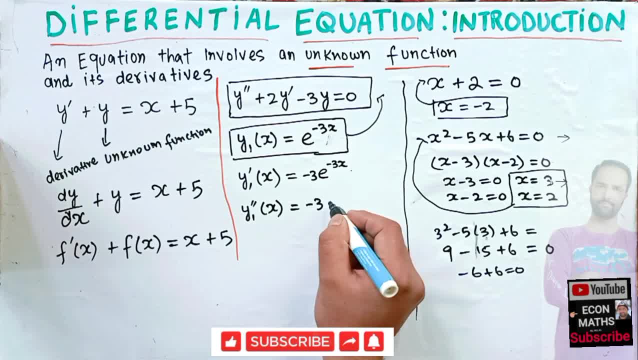 write the second derivative. similarly, we have 3 minus 3 e to the power minus 3 x as it is, and take the derivative of this exponent, that is minus 3 x. the derivative of x is 1, so we get here minus 3 by chain rule. okay, so minus 3 into minus 3 is plus 9, so we get here 9 e to the power minus 3 x. 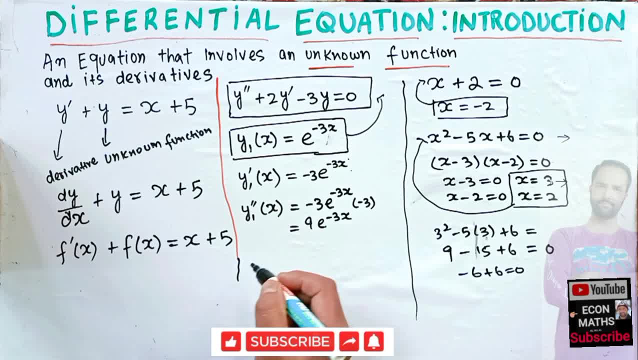 okay. so we got now to check whether this very step satisfies this equation. just plug these values, so y prime and the value of y prime is this: y 1 prime. the value of y prime is y 1 prime. so just plug these values in this equation: so y 1 y. 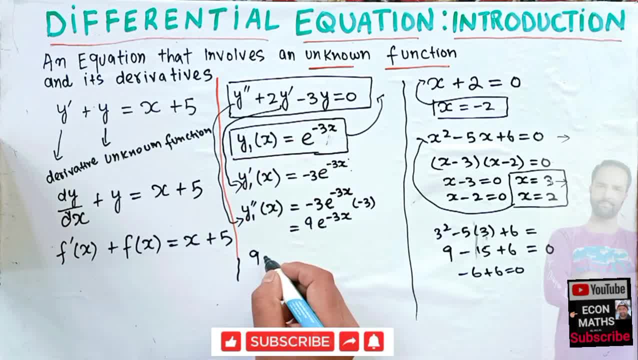 prime is equal to this very step, that is 9 e to the power minus 3 x. plus we have 2 and y. prime we got here is minus 3 e to the power minus 3 x. then we have minus 3 y, so we got y: 1 x is equal to. 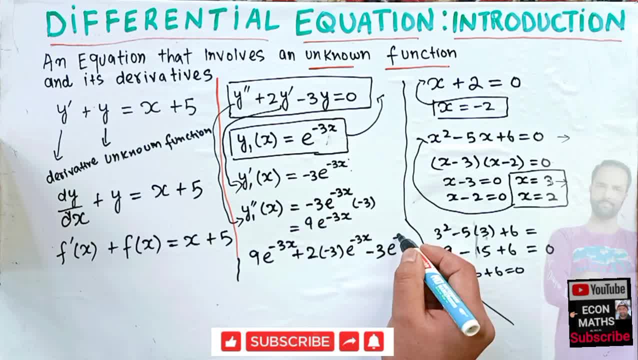 e to the power minus 3 x. okay, so this comes out to be 9. e to the power minus 3 x. so two threes are minus 6. e to the power minus 3 x, minus 3. e to the power minus 3 x, so this comes out to be 9. e to the power minus 3 x, so minus 6. 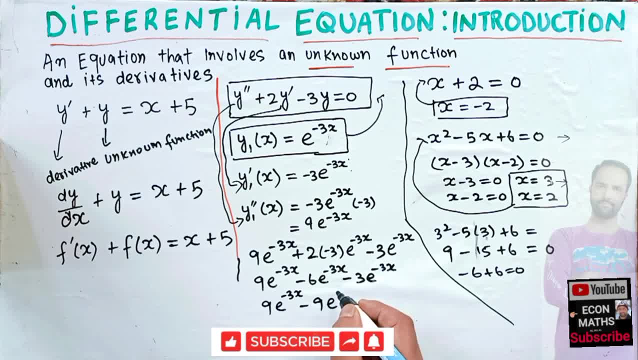 minus 3 is minus 9, e to the power minus 3 x, which of course is equal to 0 here. okay, so if we subtract these two variables here, so we will get 0. okay, we say that y, 1, x is the what we call the solution of this differential equations. okay, and how do we verify? simply, 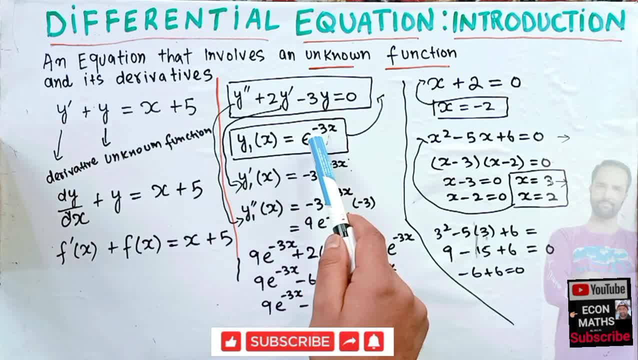 if y 1 x is equal to e to the power, minus 3 x is solution of this equation. we need to take y 1 prime. that means first derivative of this equation. okay, so if we take first derivative of this equation, that is, y 1 prime, this comes out to be minus 3 e to the power, minus 3 x. 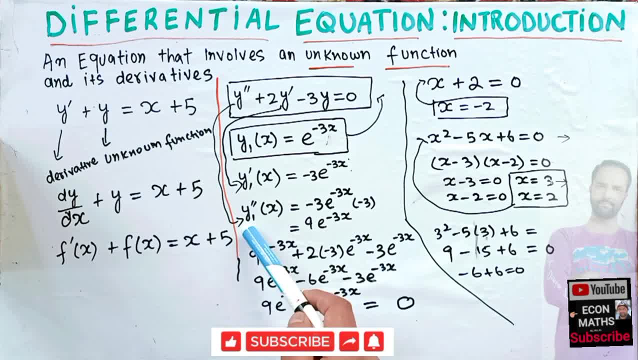 also we need to find out y double prime. that means the solution of this differential equation. second derivative of this equation which we got here: 9 e to the power minus 3 x. and when we put the value of y 1, y 1 prime and y 1 double prime in this equation we get a result equal to 0 and 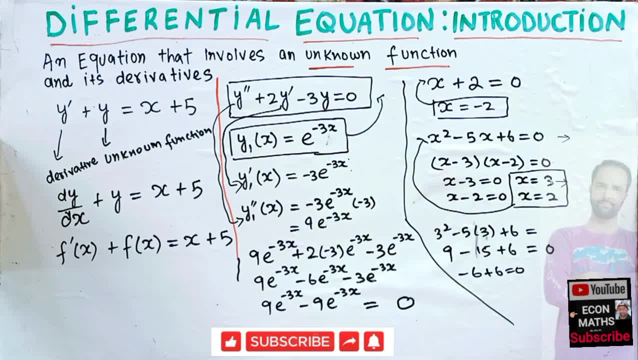 we say, oh, this is the solution of the differential equation. now, how did i get this very thing? so i, as i have told you earlier, i will explain in upcoming videos how to get the solution of a differential equations. okay, in this case we would have another setup, another function. is the solution of the differential equations? okay, so i, i can. 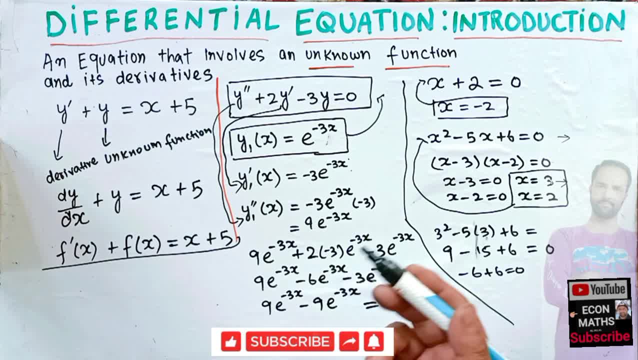 say, i will say, in fact it has another solution also. that is, if i write y 2, so just i am just differentiating it with this y 1, so i say y 2, 0, 1. this is what, welcome the y, i will called as differential equation. okay, but let's assume 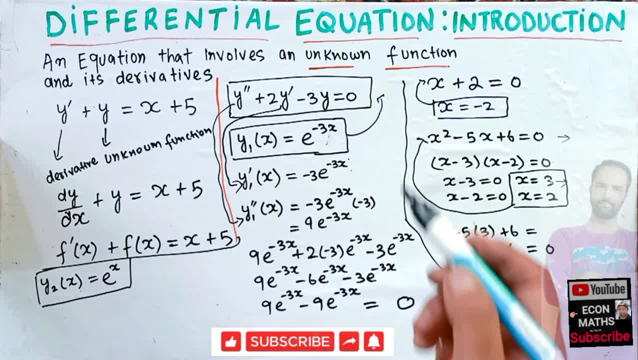 x is equal to e to the power 3: 1 of the definition of x 2 sub i 2. what is the solution of this differential equation? okay, so x 1 by 4 into y 2 is what? so if i write y 2 Megadeth minus? 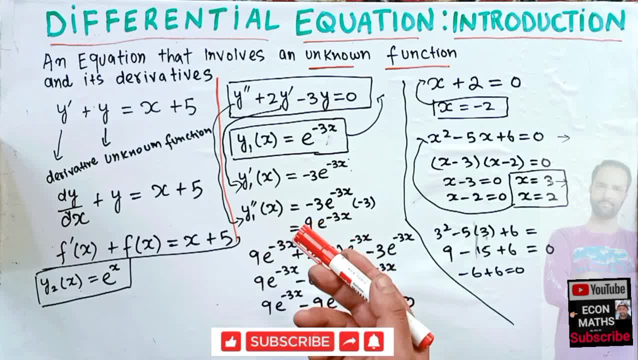 3 x 2 minus 3 x 2 in all the differences. this would be that good, okay. so the solution of this differential equation, christard, unity x2 is. i will too. your solution is actually not none of these equations. the solution of this differential equation is: x is equal to. y to the power x is also the solution of this differential equation. okay, how do i get? i will explain in upcoming videos how to get the solution after differential equation for you. since it is an introductory video, i will not have the ability to make all this stuff in this video. okay, so let's assume whole. 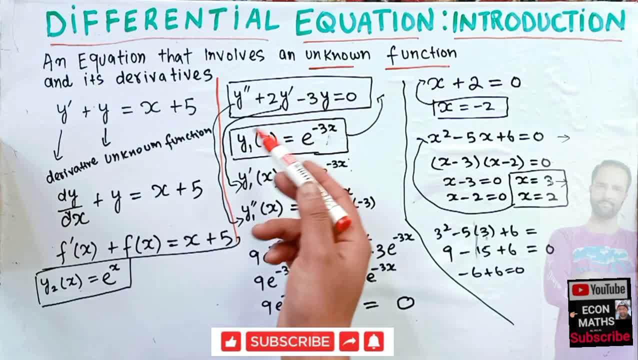 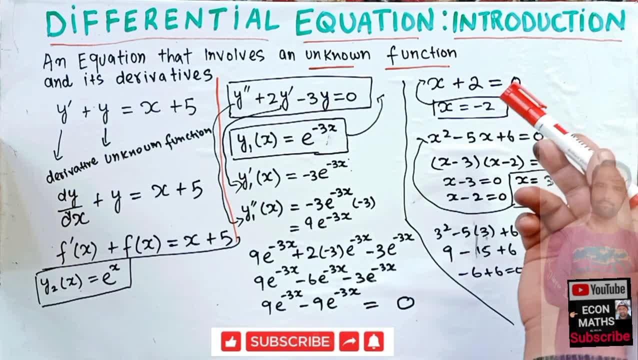 let's assume that if you are interested in, say, to be wash others for the Nineth of this equation, if this is the equation, solution of this differential equation, then so this, should this function, should satisfy this equation. also, as in case of regular equations, if we got the 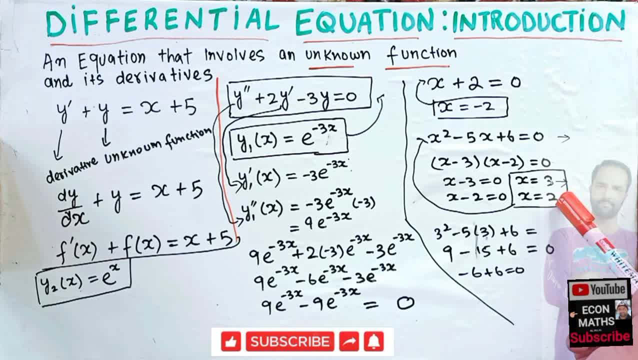 solution of the quadratic equation is: x is equal to 3 and x is equal to 2. if we put the value of 3 here, we should get this. 3 should satisfy this equation. okay, that means we should get left hand side equal to right hand side. so here we have seen. i am saying that this equation, this differential, 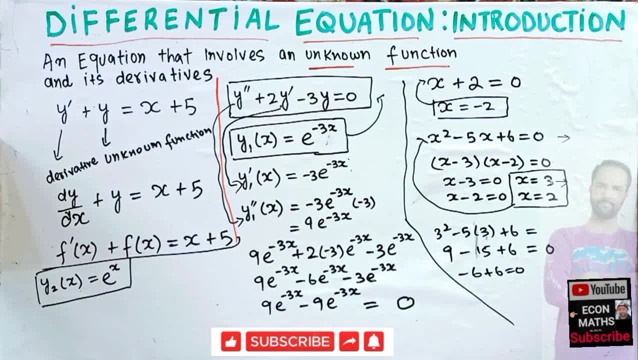 equation is another solution now to verify this simple, as we have done here. so what is our y2, y2, x, y2 prime? since we need to find this y, y prime and y double prime first, we find y prime. okay, so y2 prime comes out to be: 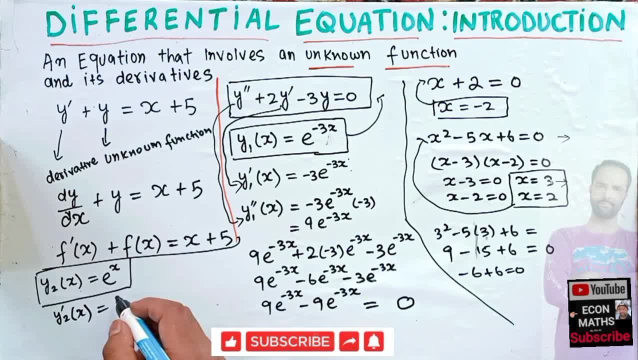 y prime and y double prime comes out to be y prime and y double prime comes out to be derivative of an exponential function is the exponential function in itself, so it is e to the power x. okay, simple stuff. derivative of x is 1, so this is e to the power x into 1, we will get. 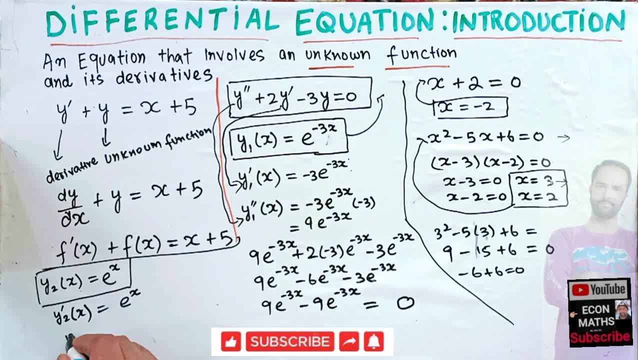 the same stuff. so okay. similarly, we need to find y to double prime x. that means second derivative of this equation, so it is a second derivative. will be also e to the power x. okay, now to verify whether this is actually the solution of this differential equation, just plug the values here. 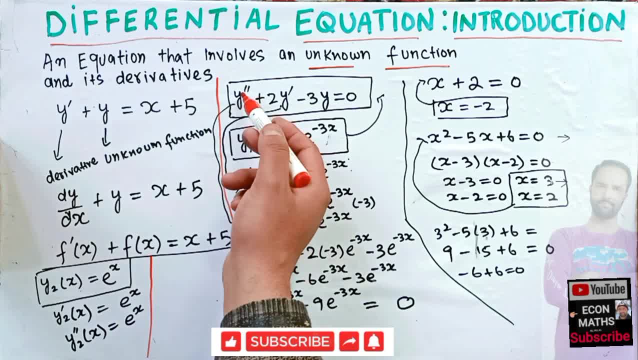 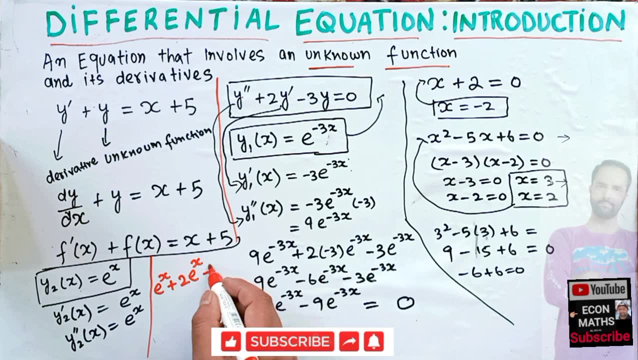 so we have y double prime is equal to e to the power x. so i can write here e to the power x. then we have plus 2 y prime. we got here y 2 prime is equal to e to the power x. okay, then we have minus. 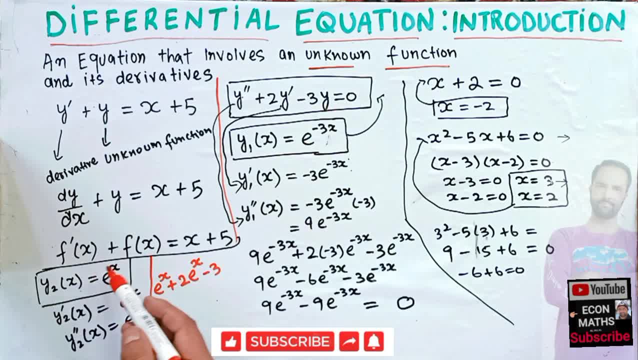 3 and y is equal to y to x, which is equal to e to the power x. okay, so e to the power x plus 2 to 2. e to the power x comes out to be 3, e to the power x minus 3, e to the power x, which, of course, is equal to 0. okay, so the point that i want to make in this 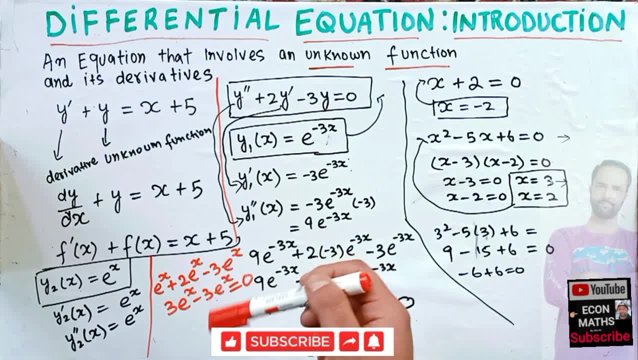 video is that the solution of a differential equation is a function. here we have seen we got this very stuff as the solution of a differential equation is a function. here we have seen, we got the solution of this differential function, or a set of functions. in fact, we got another solution. 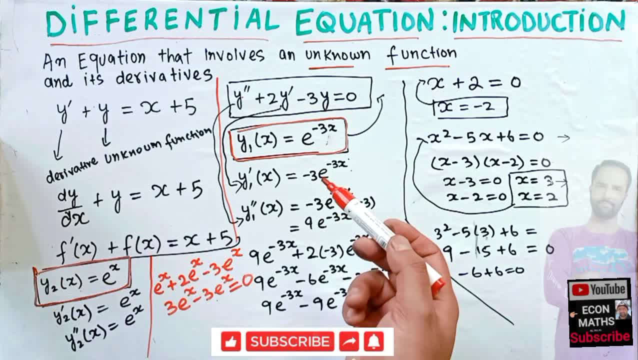 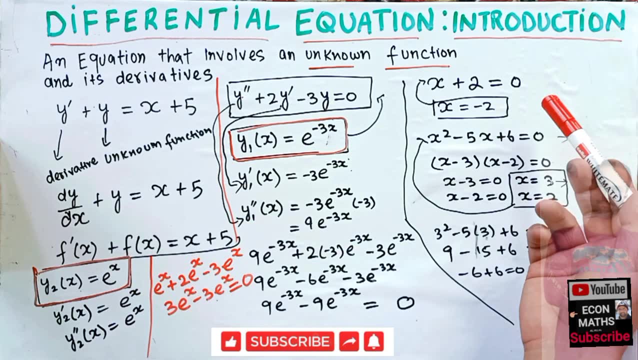 is this: e to the power x. okay, so the solution of a differential equation is a function or a set of functions, or what we call also the class of functions. okay, the difference is simple. in case of the regular equations we get the solution: a number or a set of numbers. in the first. 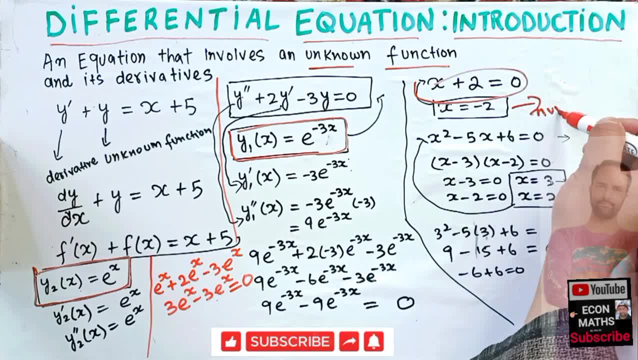 equation we got, x is equal to minus 2 a number, and in this equation we got two solutions, that is, three and two, which are set of numbers. here we got set of numbers, but in case of a differential equation we don't get the numbers per se. we get a function or a set of functions as a solution of. 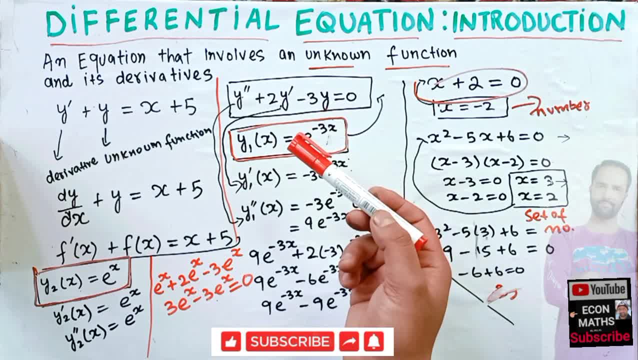 a differential equation, okay, so, um, there is another other stuff we we need to discuss. that is, what is meant by ordinary differential equations. what is order of a differential equation, whether the equation is linear or non-linear? okay, so that very discussion. we will take it into another video, okay, if the time and energy permits me. okay, so this was just.